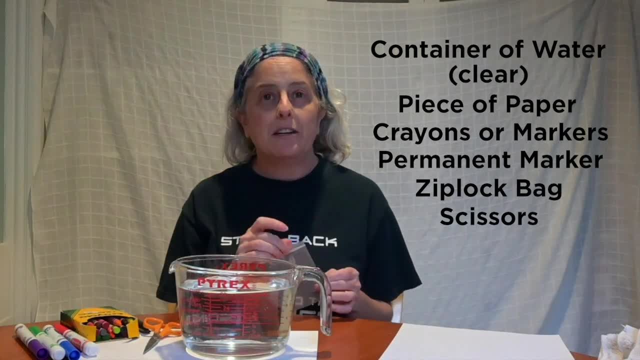 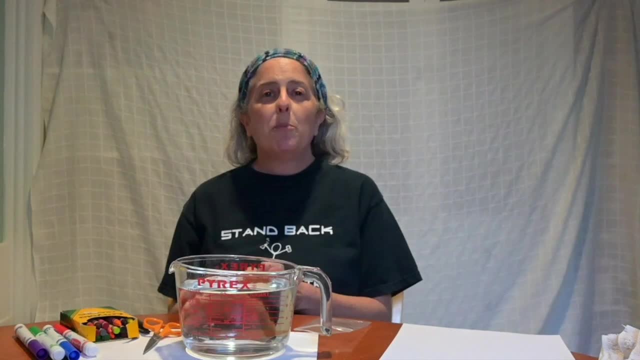 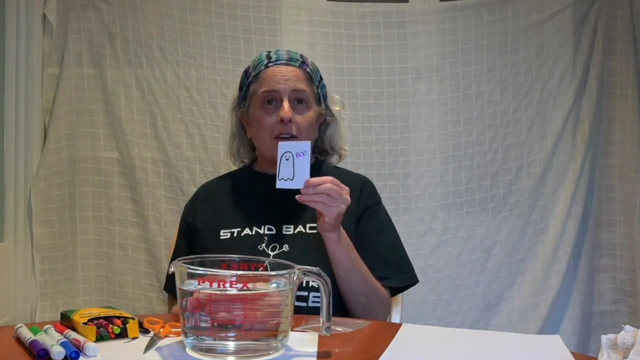 to cut your paper down so that it will fit inside your ziploc bag. So there's going to be two parts To your drawing. one part will disappear and one part will stay. Draw the entire thing on a piece of paper that will fit in your plastic bag and then fit in the water. 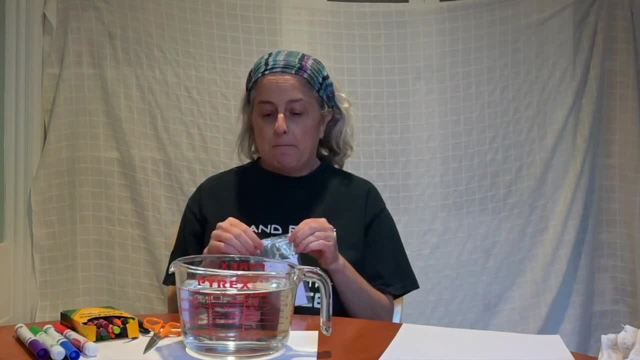 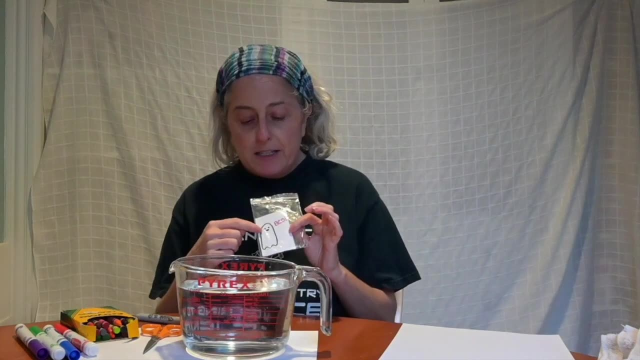 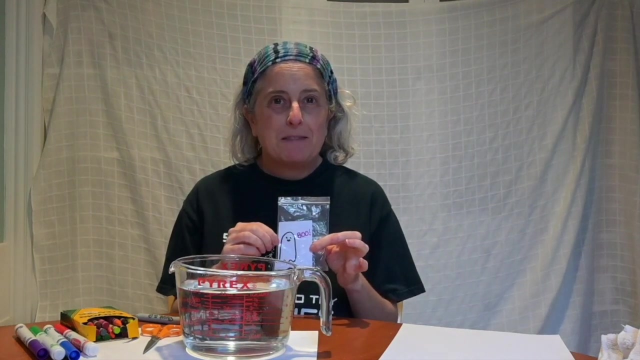 Put the drawing in the bag and seal it tight. Then, on the outside of the bag, use a permanent marker so that you can see the parts of the drawing that you want to stay. The rest of it will disappear. Let's try it Now, get ready. 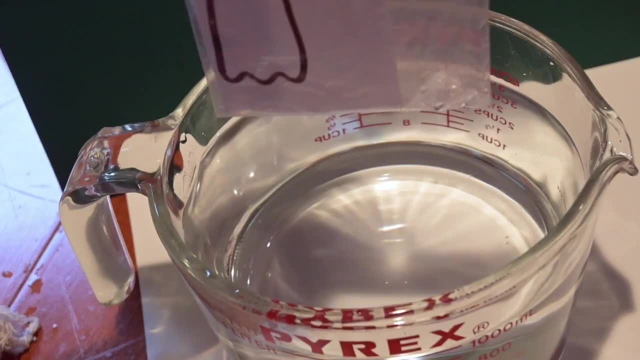 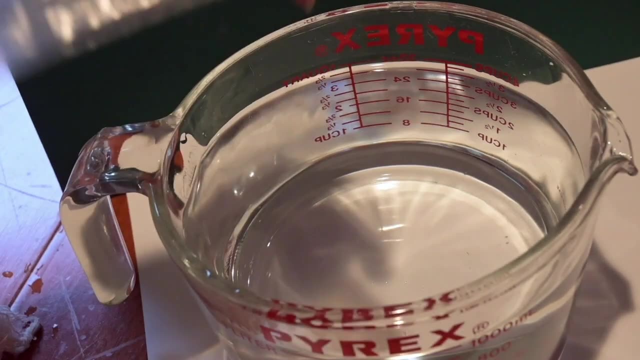 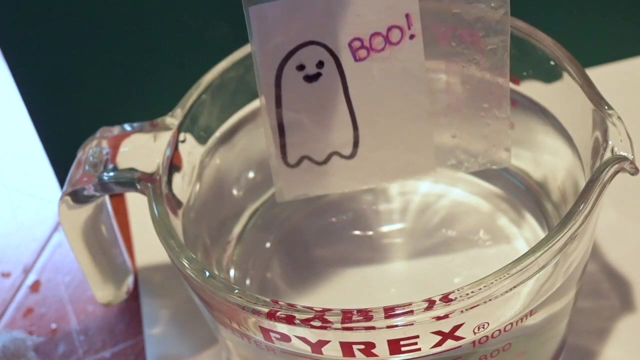 The trick to doing this is to make sure you're looking down onto the surface of the water. Don't look on the side of the container. Look from the top down, Let's see what happens. Oh, my Look down, He's gone. 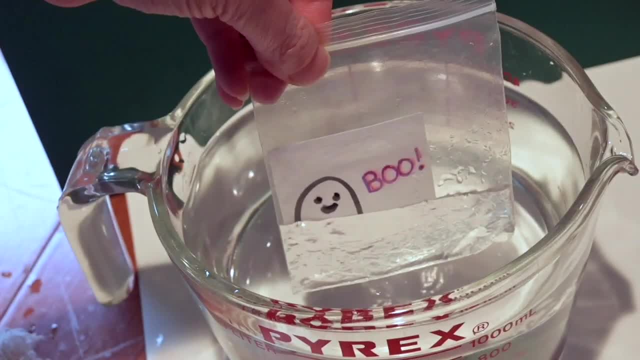 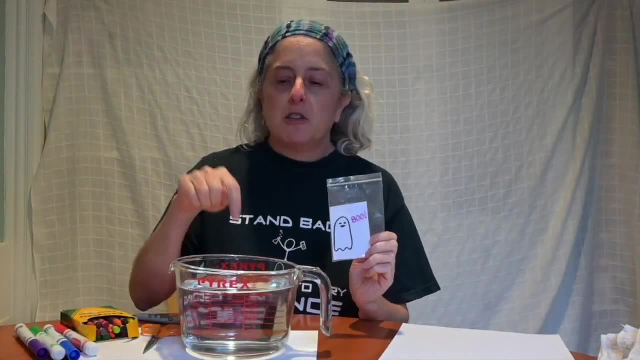 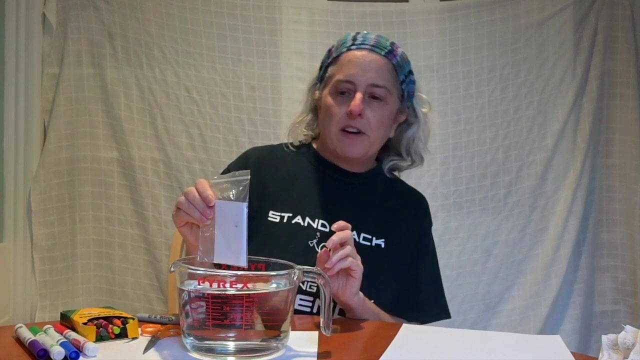 Let's try it again. If you're having trouble with this, make sure you're looking down into the surface of the water. If it doesn't work, when you put your bag up, just change your angle a little bit bit, Get a little closer, a little higher up, Just keep fussing around. It'll work. 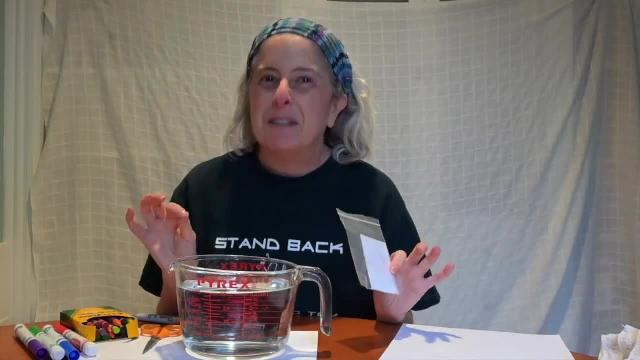 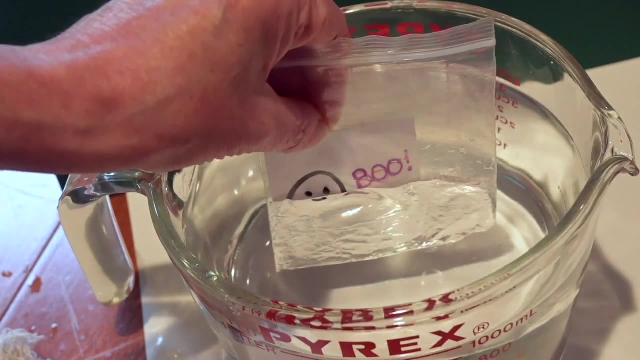 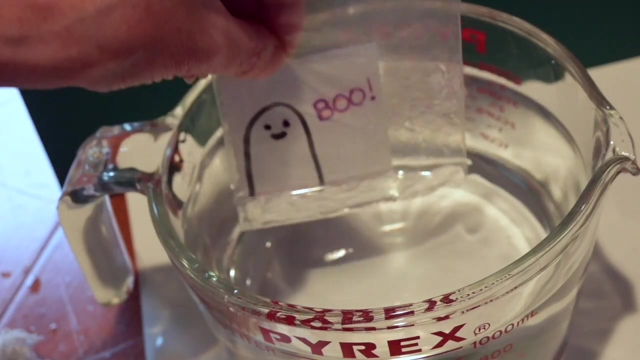 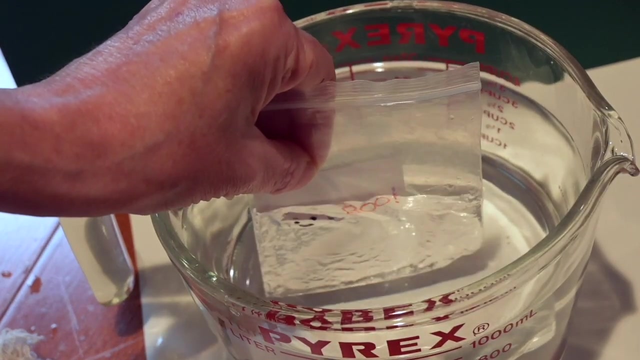 for you eventually, And when you do, it's really cool. So what's happening here? In order for you to see, light needs to come into your eye. But what's happening here is the light is going into the bag and then it's getting reflected inside the bag and 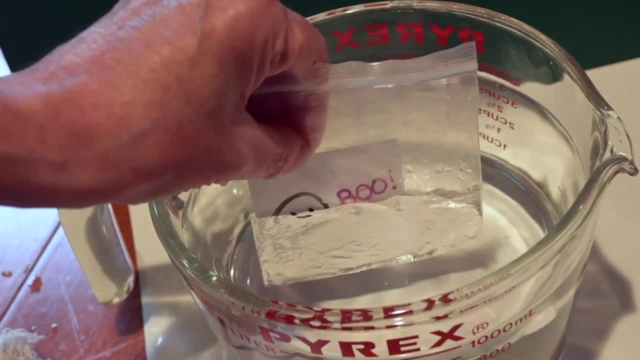 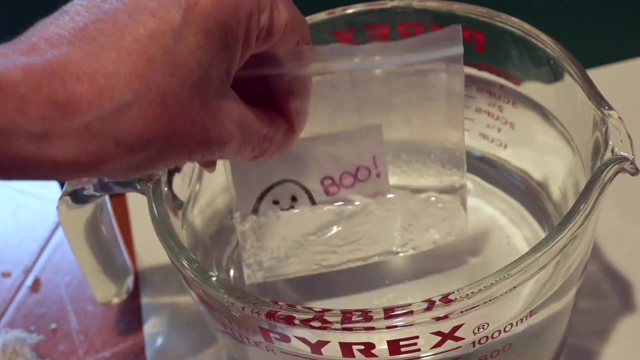 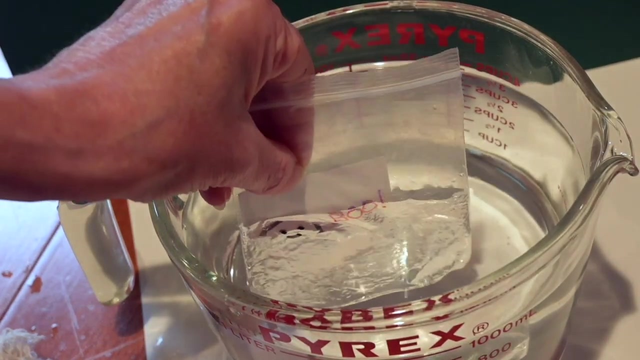 just bouncing back and forth in the bag So it never comes back out to your eye. So the ghost disappears. You can see the ghost's face and the word boo, because those are on the outside of the bag. So that light is coming out of the bag.